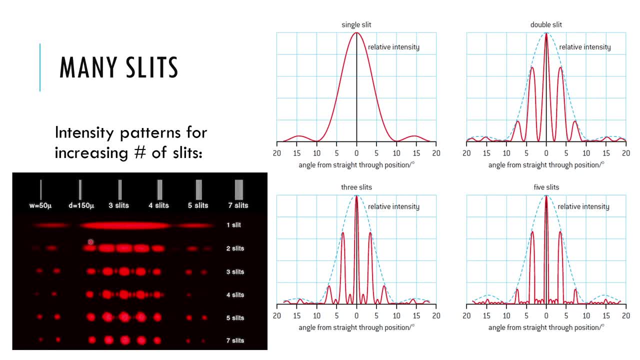 graph essentially gets focused and redistributed And so these bright spots get narrower, they get brighter and they stay the same separation apart. So we get these very narrow, very bright spots, A diffraction grading. you just add a whole bunch of slits and you make these points really, really, really small, to the point that they 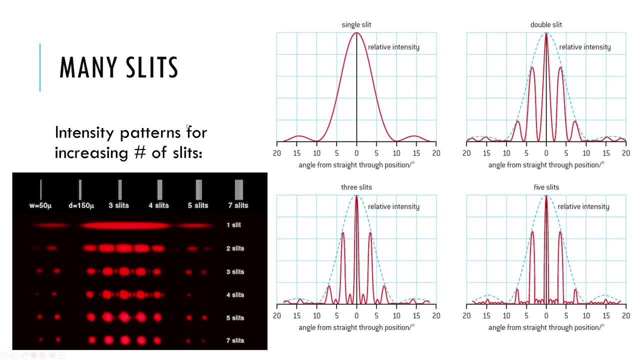 look like just pinpoints of light, All right, but those are the patterns of single slit and double slit that you absolutely positively, definitely want to know. for the IB They love like this graph especially. You really want to know the double slit pattern, And so multiple slit is very similar. 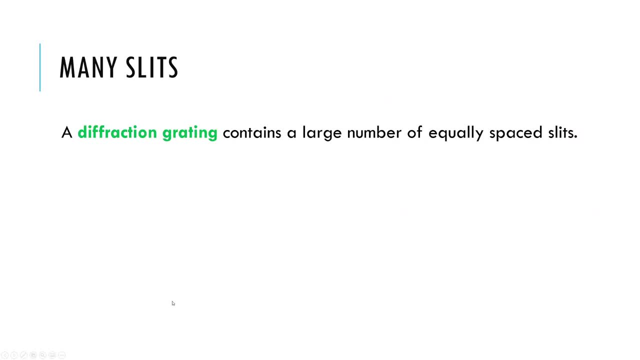 but you just get them narrower and brighter, All right. So that's what a diffraction grading is. It has a lot, way more, than five, of equally spaced slits, And the key thing with a diffraction grading is they're usually very close together. 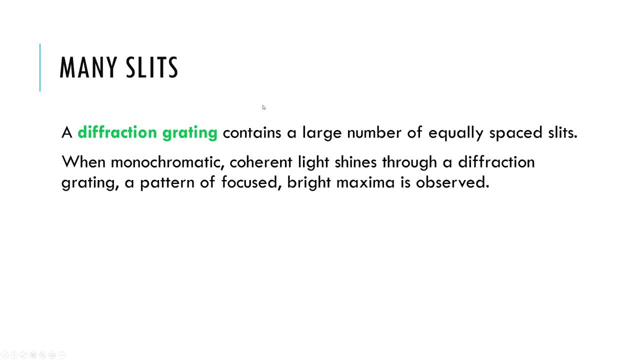 much closer than like in a double slit or anything like that. All right, so of course we're going to get very bright focused maximums. That's the idea. We'll look a little bit very briefly at the kind of geometry setup of this. Again, it's all about path difference. 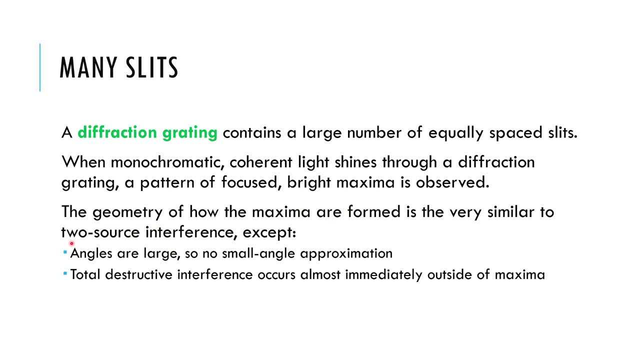 and thinking about that in terms of wavelength, But so it's very similar to two source interference. The only difference with diffraction grading really is that we're not, we can't- do small angle approximation anymore. The kind of point of a diffraction grading is to spread. 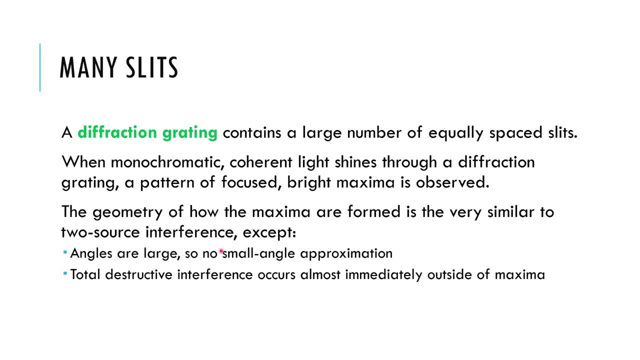 light out a lot, based on its wavelength. We want big angles, And so we put the slits very close to each other, usually by scoring some kind of material, And so the angles are going to be big. so we can't call sine of theta about equal to theta anymore. All right, and what we see is that there's 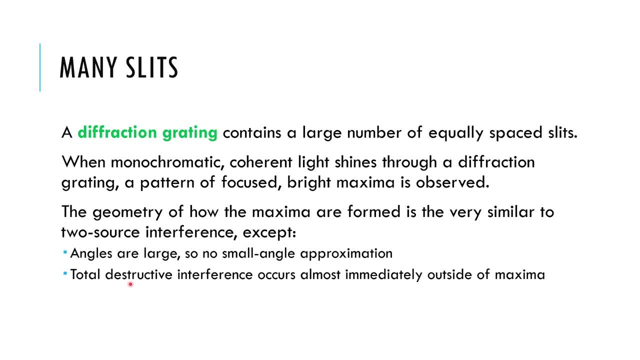 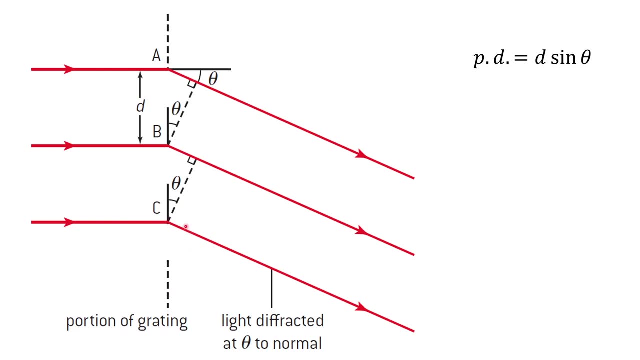 total destructive interference immediately outside of our maxima. So the bright spots are very bright and right outside of the bright spot it's totally dark, which again is kind of the point. You want to really separate these colors by wavelength. Okay, here's a picture of a sketch of a diffraction grading. 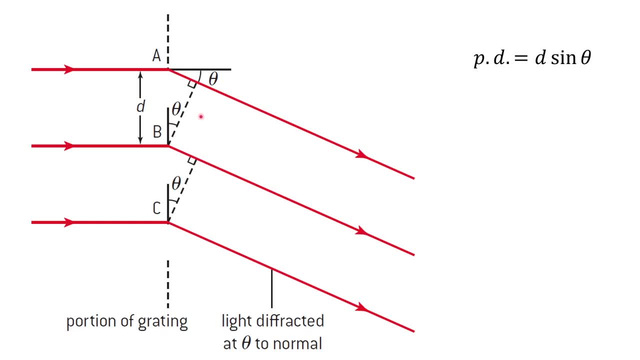 So here you see all these little kind of openings, and we're just looking at a few of them. But again, the same exact idea. Here's like a portion of the grading right. There's many, many, many, perhaps thousands of slits. But so the light gets diffracted and let's say we have 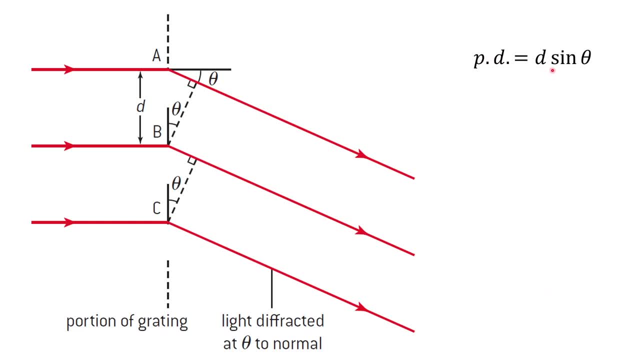 some maximum down here that we want to think about. So we can look at the path difference Just like before. this is where the setup is the same. The path difference is d sine theta, where d will be the spacing of my path. So we can look at the path difference. 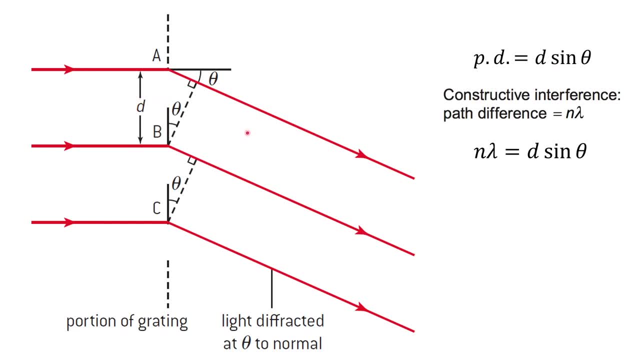 We can look at my slits, the separation between slits. That's just how the geometry works out. This is how much further this ray has to go than say this ray to that maximum All right, and constructive interference, remember, will happen when the path difference is an integer. 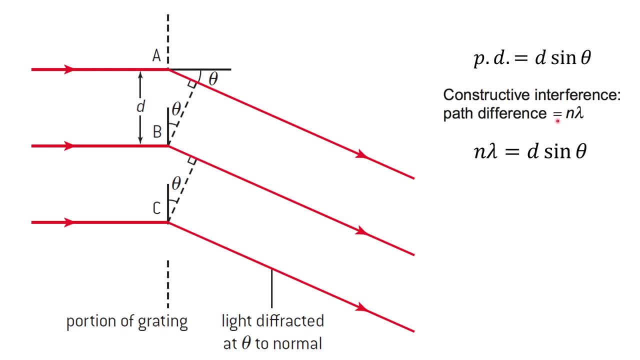 number of wavelengths. So one wavelength or two wavelengths or five wavelengths, If the path difference is an integer number of wavelengths, you get constructive interference. So the equation we're going to come up with is set them equal. All right, With the diffraction gradient. we typically name n the order. 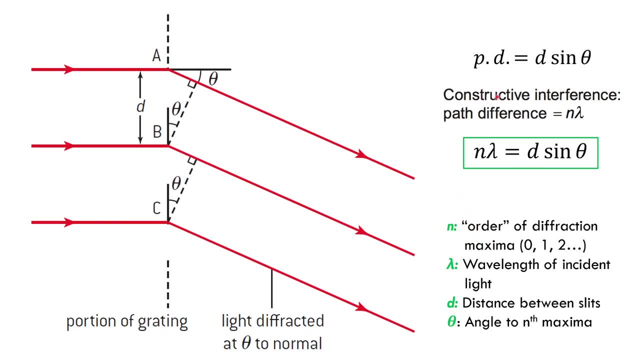 We're going to look at what we call the order of the diffraction maxima. So there's a zeroth order and a first order and a second order, maximum. So we'll look at a picture of that in a second. that, I think, will help. 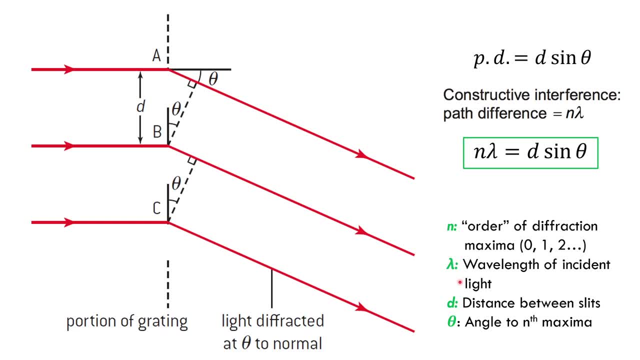 As always, lambda is the wavelength of the light coming into my grading here. Little d is the same as it was before. It's the distance between the slits, And theta is the angle to the nth maxima. All right, so I can find the angle to the. 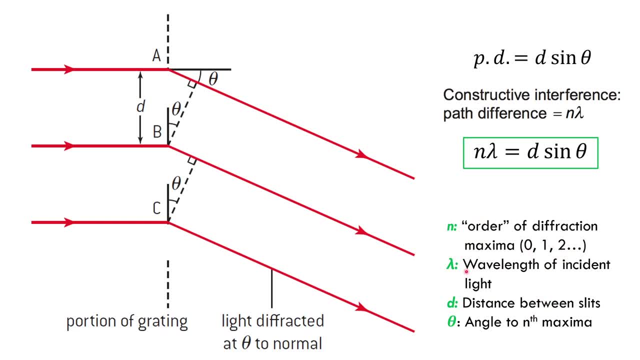 first maximum or the angle to the second. Notice: if n equals zero, the zeroth order, the angle will always be zero. Right, That's how I would get that. The sine of zero is zero, But everything else, n equals one, n equals two. my first bright spot outside of the middle: 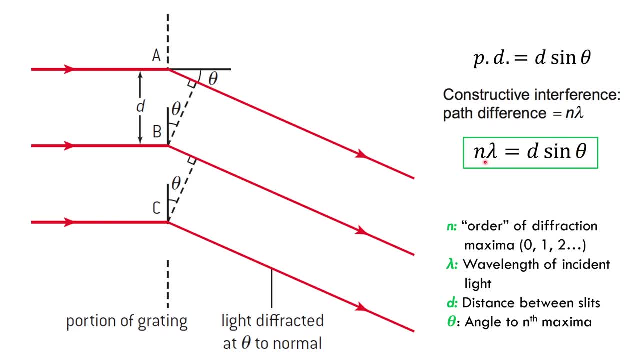 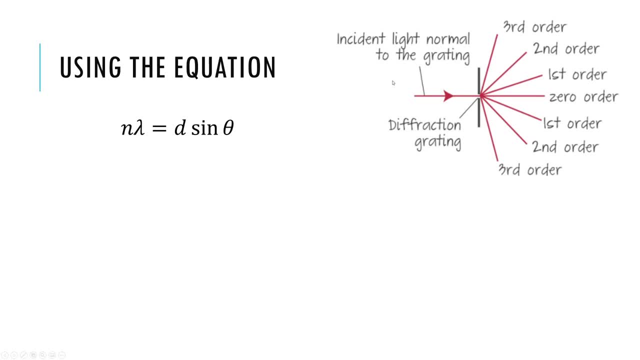 my second bright spot outside of the middle. those will have different angles depending on, say, the wavelength of light and the separation of your slits. Okay, this is essentially what you get when you shine light through a diffraction grading. Some light shines straight through forms that central kind of pinpoint of light. 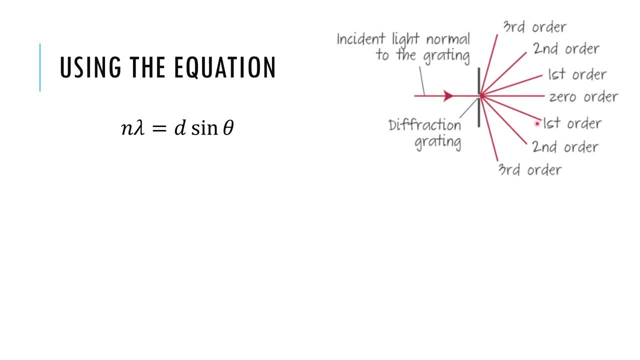 that zero order maximum. But then you're going to have. this is how we label them, so be careful. This can be a little confusing, But these will be n equals one, these will be n equals two, these will be n equals three. So my second order, for example: maximum. 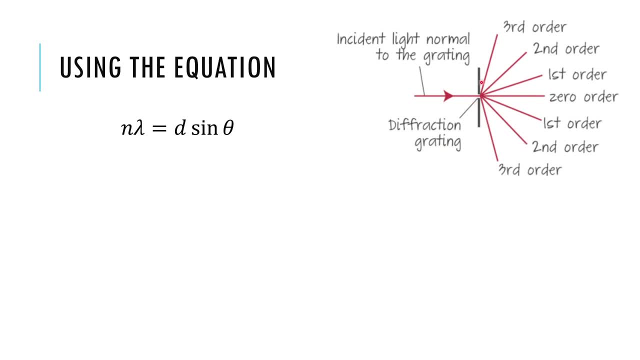 over here and over here. One question the IB loves to ask you about- in fact, we'll try one at the end here- is: how many maxima will you see? Because these angles are big. you can look at this picture here and imagine if it's spreading out like this, you won't get a fourth order maximum. 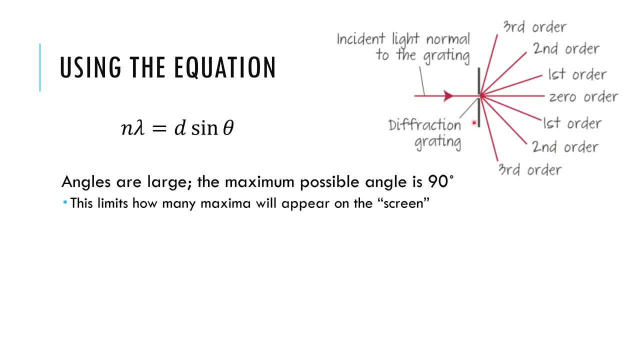 like in this setup. It would have to go like this: maybe to get to that fourth order and you can't diffract more than 90 degrees, or else you're not going through the diffraction grading anymore. So because the angles are so big, there is a limit to how many of these bright spots you're gonna see. 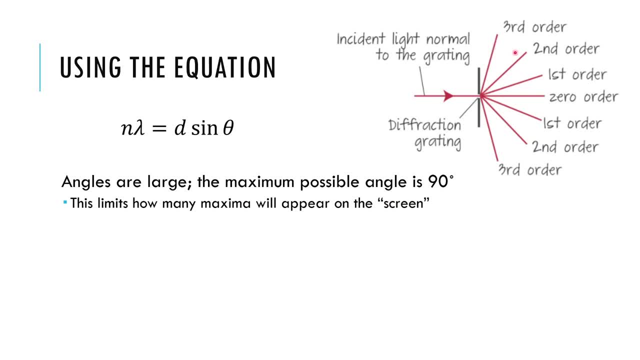 And so they like to ask that question: how many will you see? In this case, it would be: let's see one, two, three, four, five, six, seven bright spots you would see on the screen. All right, so a maximum possible angle of diffraction is 90 degrees is a good tip to remember. 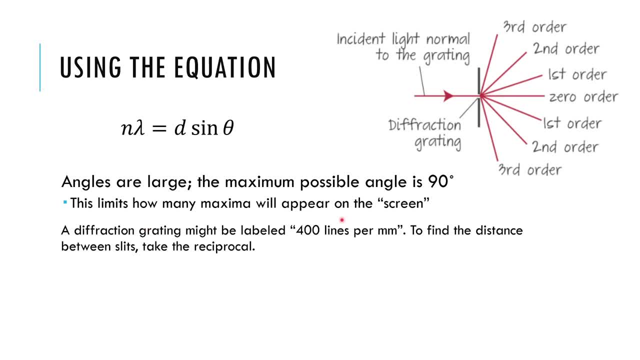 The other thing that you'll see a lot is this kind of thing. You might play with these in class. The diffraction grading will say something like 400 lines per millimeter or 12,000 lines per inch, And you'll see that there are per unit length. So they're very, very, very again scored. 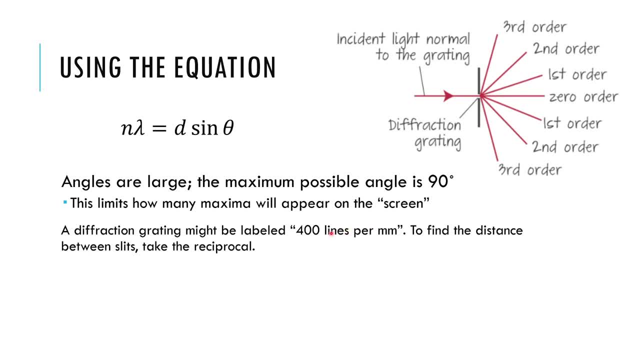 like very, very tight together. So just think about what that means. If there's 400 lines per millimeter, the distance between each line must be one over 400 in millimeters. So you take the reciprocal of that, because you gotta use your physics brain here and think about: okay D. 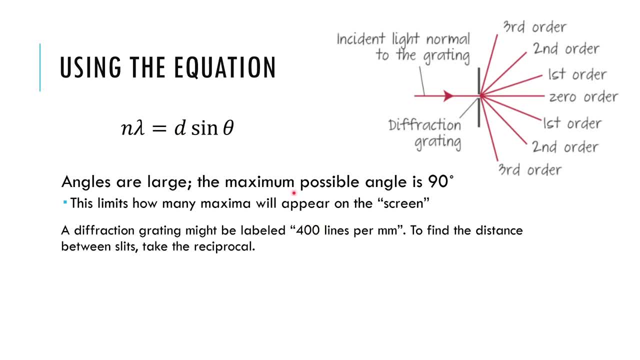 what I want is the distance between two adjacent slits. If I know there's 400 in one millimeter, I better divide one by 400.. All right, here's a kind of formal factor label-y kind of way that you could do it with some. 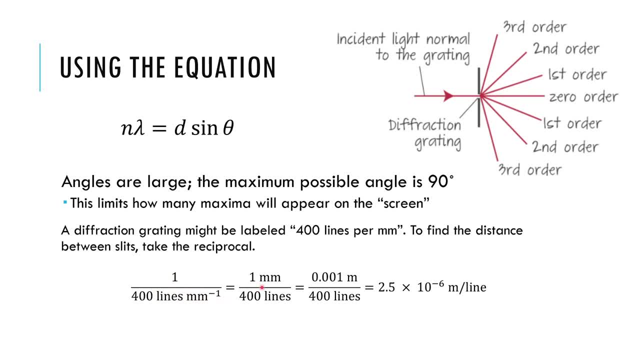 dimensional analysis, One over 400 lines per millimeter. So I got this many millimeters and 400 lines. Convert, convert, convert And you should find that there's this spacing between each line, In other words, that's the spacing between the slits. So we would call that little D. 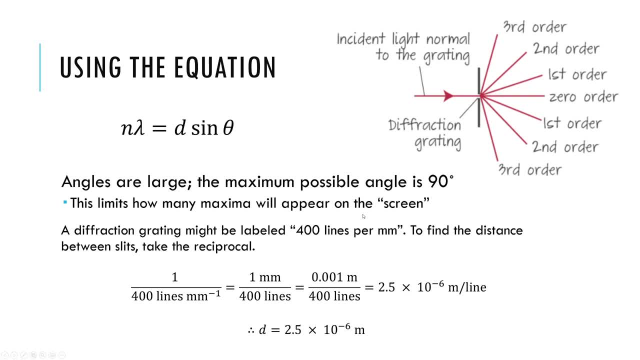 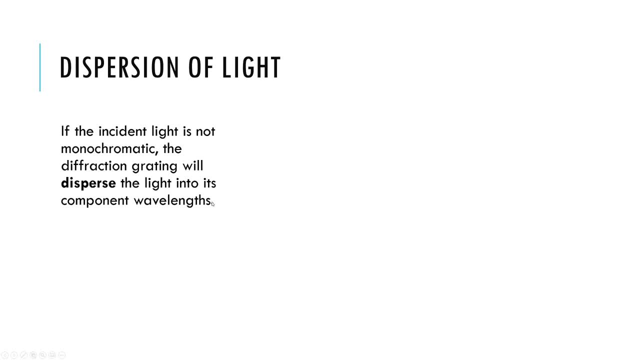 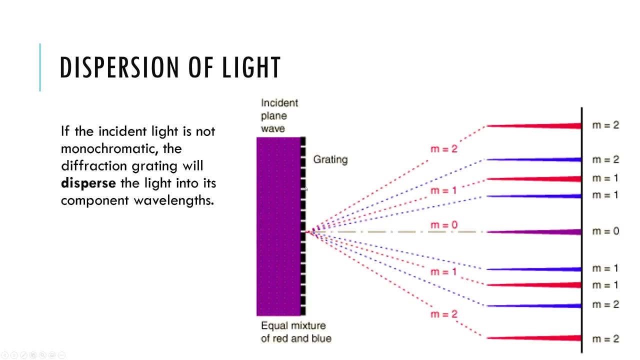 All right, this is just an example number, but that's a very common thing that you'll see in these problems. Okay, One of the main uses for a diffraction grading is to disperse light. Remember, dispersion means to break it up into its component wavelengths. 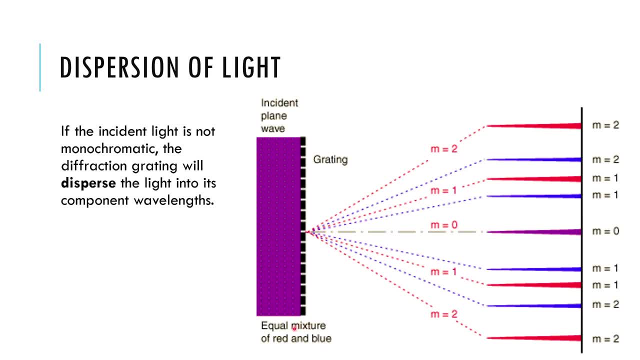 So here's an example of purple light, Purple which is an equal mixture of, let's say, red and blue light combined together. When red and blue hit your eyeball at the same time, your eye goes whoa, let's call that purple. And so there's that purple light shining through, because at 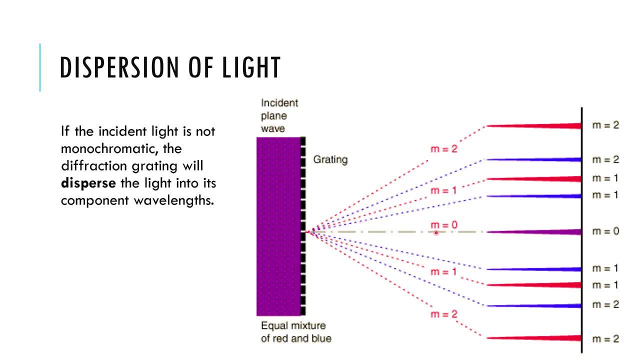 here in this picture they're using M, but that's what the IB is calling N At that zeroth order maximum. the angle for red light and blue light is both zeros, So they'll still be purple here. But for N equals 1 in my first order maximum. 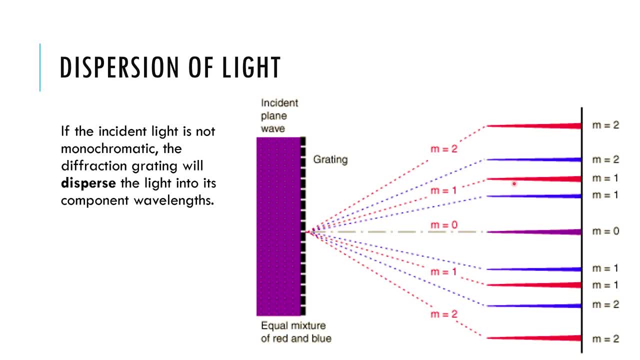 if you can look at the equation and convince yourself of this. you definitely want to know red and blue, which one has a longer wavelength, But red should get bent at a greater angle than blue, if I use that equation Right. And so the red will get meant at an angle higher than the directionnia of red time, and so the red 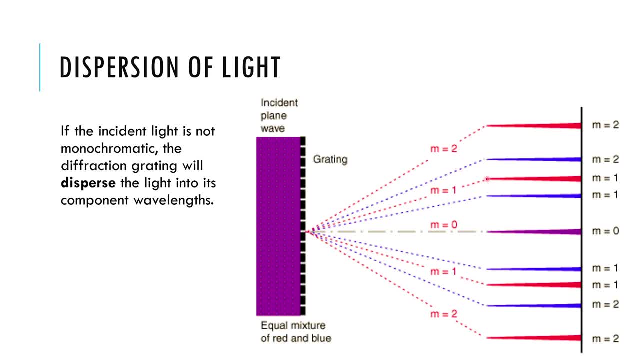 will get split up from the blue. so you'll see that this purple light is indeed made of red and blue light. It would shine purple in the middle and red way over here and blue over here, so you could see the different pieces that make it up. Many different points. 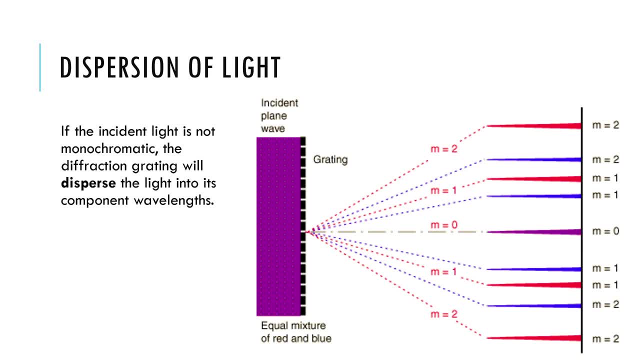 in physics, when we're studying especially atomic physics or astrophysics, we really are interested in seeing what different wavelengths make up a source of light. It can tell us a lot about chemical composition and all kinds of other stuff. That's what we use it for: analyzing gas, spectra, stars, elements, all kinds of stuff. 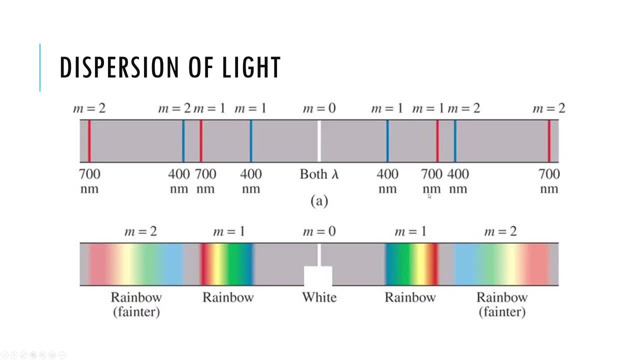 A lot of it, which we'll study later in the course. Here's another picture that just shows the same kind of thing. This is again that idea of purple light being split up into blue and red. If you have white light shining through a diffraction, grating white light, remember. 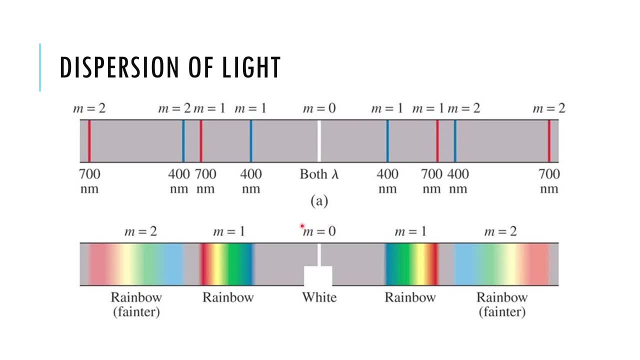 is made up of all of the colors of the rainbow and then some. It's probably also infrared in the light, And ultraviolet and so on and so on. But of the stuff we can see, the visible spectrum will be smeared out. then The red light will get diffracted at a great angle. The blue 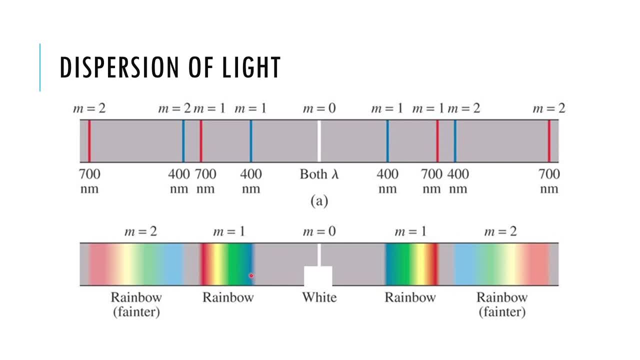 light will get diffracted at a not so great angle And the OIGB will get diffracted all in between. The green light will get diffracted by a medium amount, so depending on its wavelength it gets spread out different amounts. You see white light dispersed into all the colors. 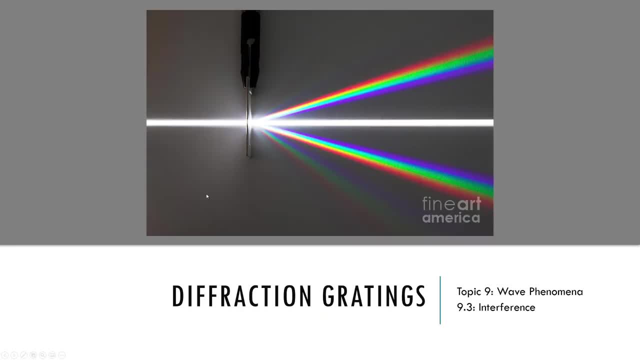 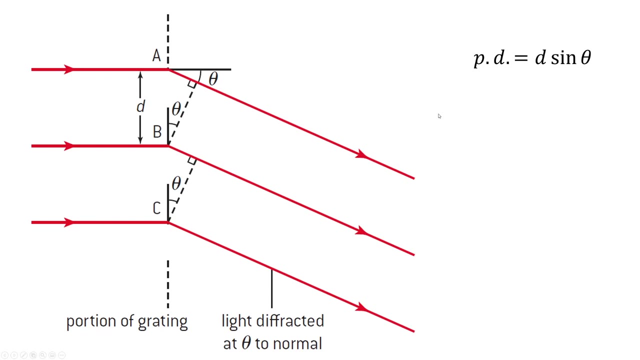 of the rainbow with this kind of thing. Here's a picture And again, we'll definitely play with this kind of stuff in class if you haven't seen it already, But you can really. if you look through one of these things at a source of white light, you see that rainbow being split out from the source of light. 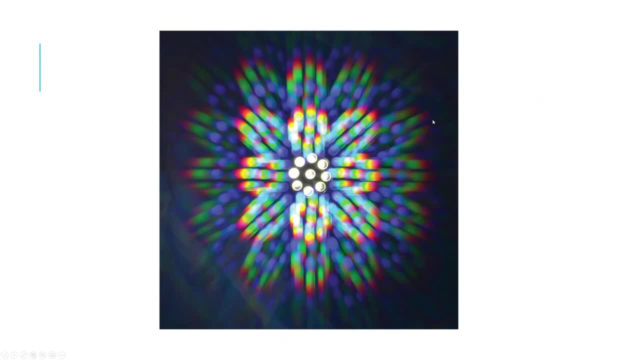 All right, And last, here is a little. here's another picture, Same thing. This is what you would see if you look through a diffraction grating at like this is a flashlight or something, an LED flashlight, So you can see the light is being spread out red, a lot The. 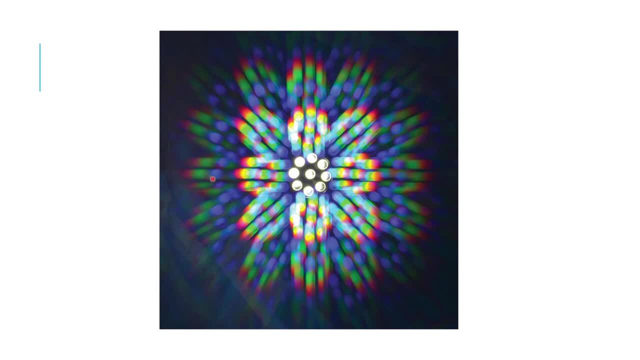 blue not so much, And over here in the second order, it gets even more extreme. If you can look at the equation, think about why that is. The red gets spread out a lot, The blue not so much. You really see all of the colors that make up this white light. 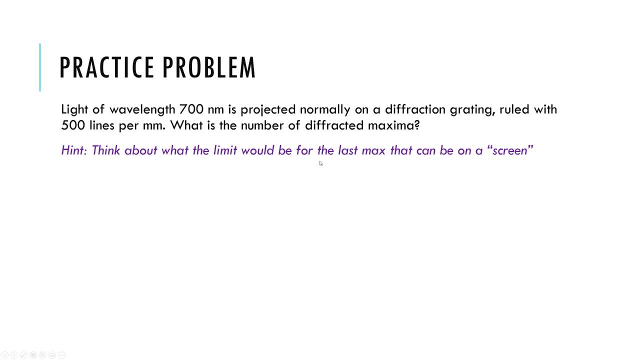 Okay, Here's a problem for you to try. Take a moment, pause it and see if you can't do this with those methods and techniques. we talked about This last part. you will especially need to think about what a reasonable answer is based on the math that you do, All right. 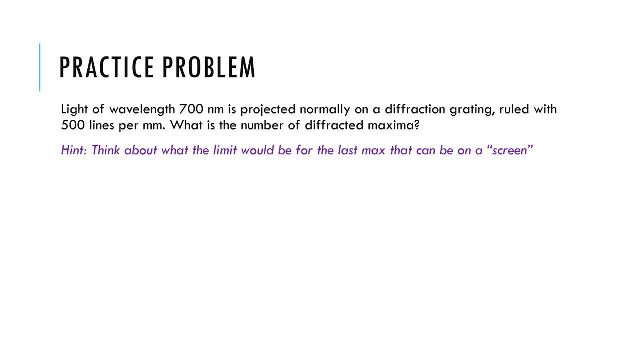 So give it a shot. Pause the video 1. Okay, Here we go, The answer, the solution. here. of course, we want to use our diffraction grating equation And the idea is: I want to solve for n: What's the number of diffracts? 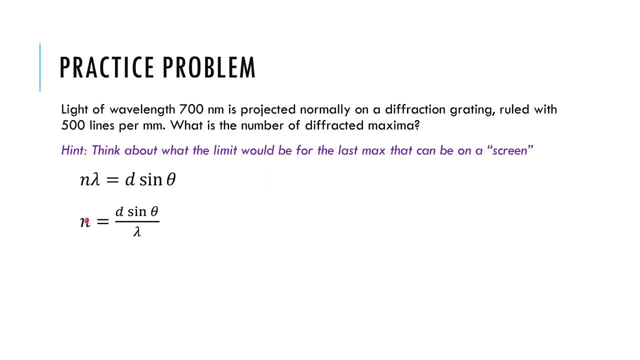 in maxima. So in other words, I'm kind of solving here for the order that I get at a certain angle. So the order that I get at what I'm going to do in a second is put in 90 degrees Because, remember, that's the maximum, That's the cutoff. 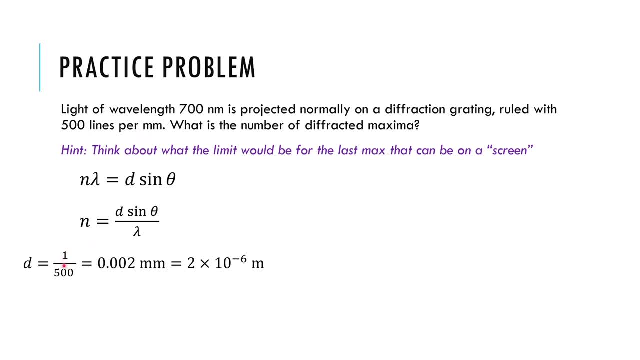 Let's deal with this first. I have 500 lines per millimeter, so I know I got 1 over 500 millimeters in between each line, So .002 millimeters will be my spacing, a little d, Or in other words 2 times 10 to the minus 6 meters. All right, So now I can start plugging. 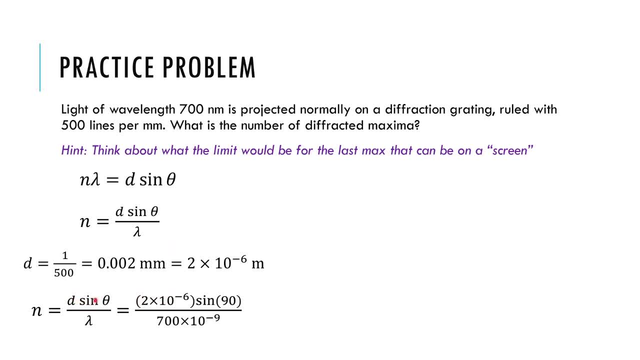 things in. That's going to be a little d. I'm going to take the sine of 90 because I to know if I look 90 degrees. so here's my diffraction grading. if I look all the way to the side, what's the last order of diffraction that I can see? possibly